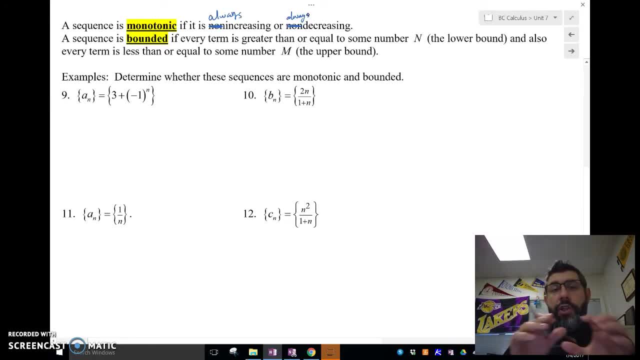 A sequence is bounded if every term is going to be either okay. if it's bounded below if every term is bigger than a certain number, and it's bounded above if every term is less than And if it's in between, meaning it's bounded above and bounded below, in between two things. 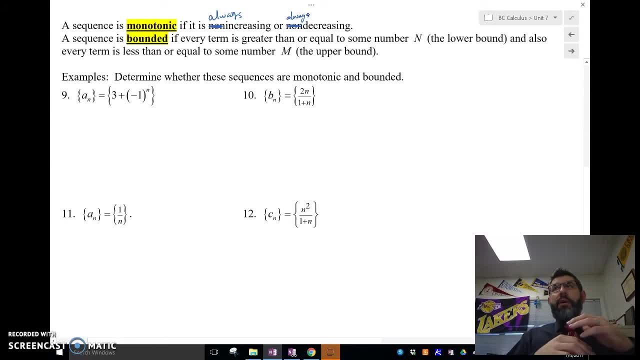 then it's called bounded. I'll show you an example and I'll kind of go through real quick where it's bounded above and bounded below and so forth. So here for this one. we've seen this one before. This was the one that was in the last video. it went two, four, two, four, two. 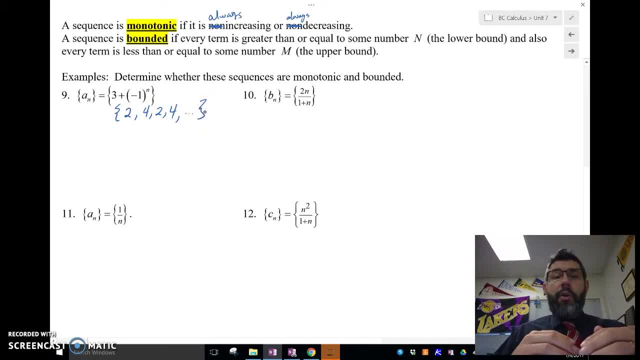 four, and so on. And this one goes two then four, then two, then four, then two, then four then two. So it's not always increasing and it's not always decreasing. So this is not monotonic. 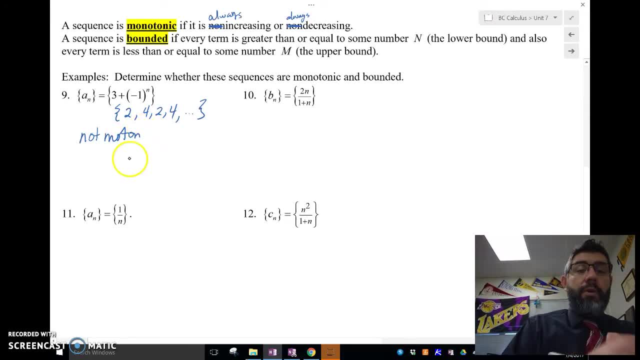 Monotonic, ton, mono, monotonic, mon, what that says moto, moto-onic, monotonic. Okay, not monotonic, But notice that it is bounded above by four. right, It's not going to get any higher than four, So it's bounded above. 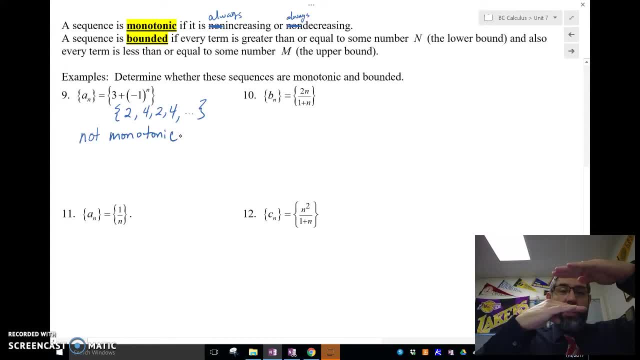 by four, and then it's never going to get lower than two. So it's bounded below by two. So since it's bounded above and bounded below, this is bounded All right. So what about number 10 here? So if we write this out, 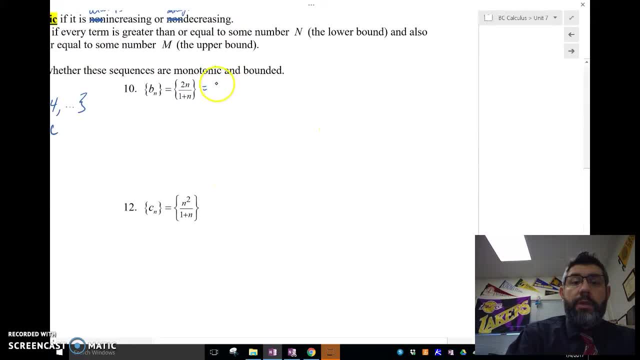 this is going to be one, and then four-thirds, and then six-fourths, and then eight-fifths, and then ten-sixths, and so on. Okay, Now notice that this is the smallest value that this is going to be. 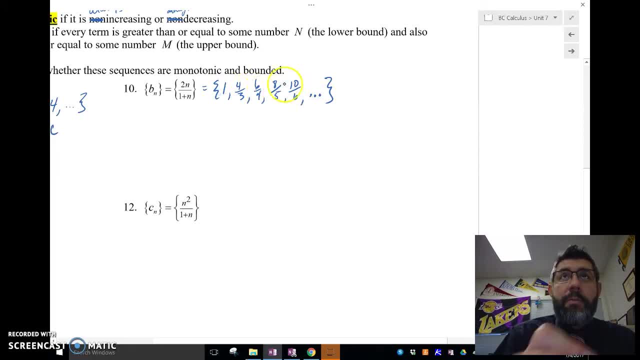 is going to be one, because these get bigger. See this, these get bigger and bigger and bigger, right? Ten-sixths is five-thirds right, So they're getting bigger, And if you remember, here, the limit as n approaches infinity. let's first talk. 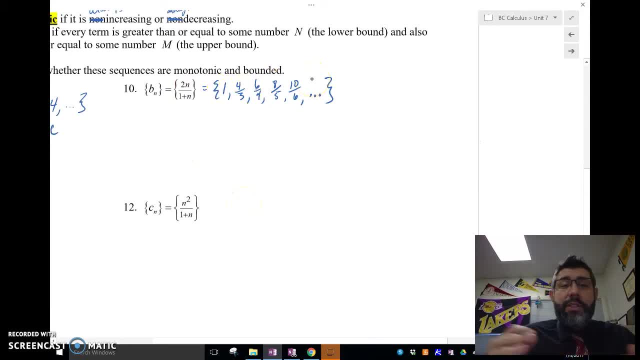 is it monotonic? Yes, it is, because it's always getting bigger. I just said it's always. it's always increasing. So this is monotonic. Now, it's always increasing. It's never going to get bigger than right It's going to. it's never going to get smaller than one. So this is. 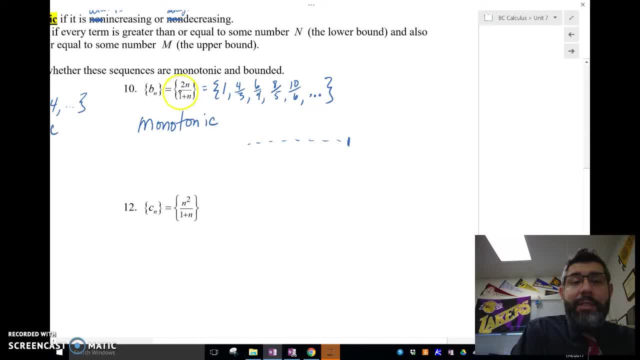 going to get bigger than one. One is where I start from, And then if I as L as the limit as n approaches infinity, here it's got a horizontal asymptote of two. So this is actually not going to get any bigger than two. This is going to kind of keep going and go closer and closer to two. 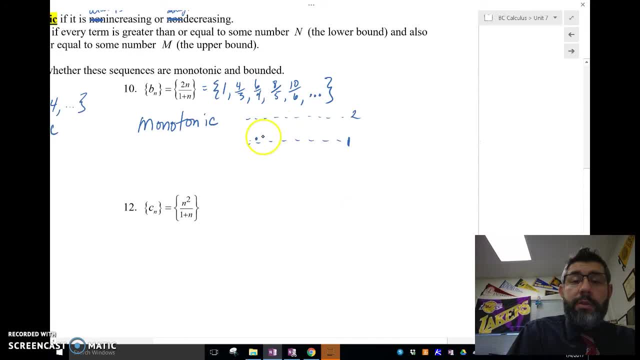 So this sequence- and I shouldn't draw a line, a sequence, you know are dots- A sequence is going to this, one's going to go to two. So this one is bounded. It's bounded above by two and below by one, And if you notice that any, you should kind of see here that a. 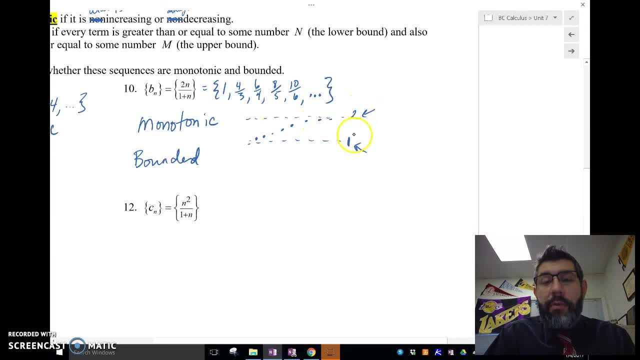 monotonic sequence that's bounded above and below. so that's bounded, is going to converge. It's going to converge to this, this value here, Or maybe not. maybe it's converging less than that, I don't know. but we know that it has to converge anyway. There's a theorem that says so. 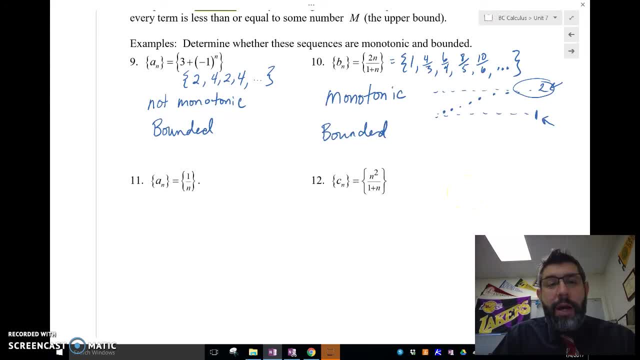 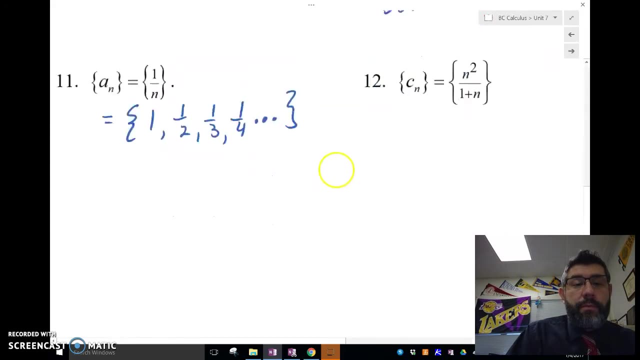 Basically, it says that any sequence that's monotonic and bounded must converge. So let's at this, one, one, one half, one third, one fourth and so on. so this function- uh, i'm sorry, function, i don't want to say function- this sequence. this sequence is monotonic, and it's monotonic because 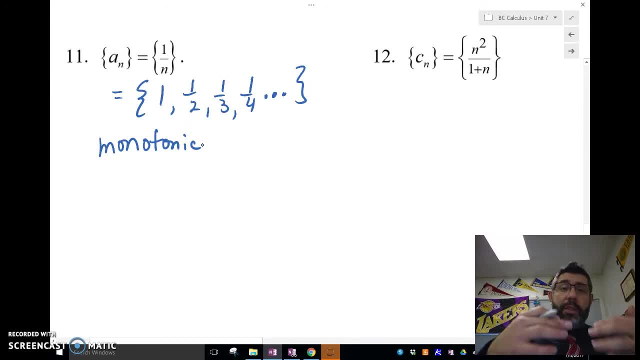 it decreases. right, it's one, then one half, then one third. it's always going to be smaller each term, and notice that the highest value it's going to be is one, and these are always going to go down, but they're never going to get past zero, like this is always going to be positive, so 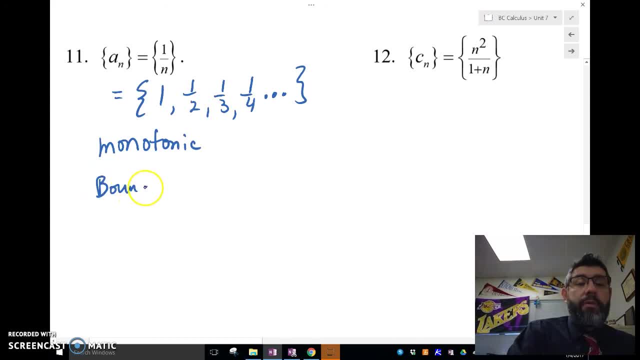 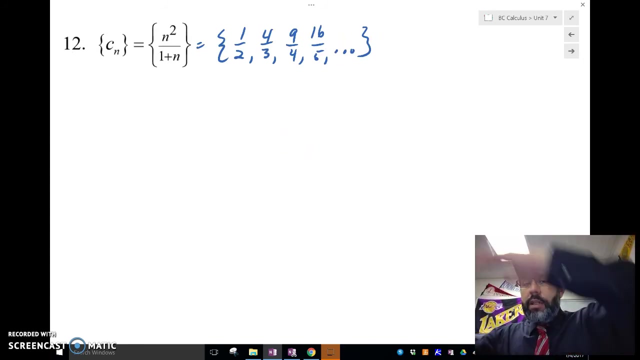 this sequence is bounded. it's bounded above by one and below by zero. all right, last one here. let's write this guy out: one half four thirds, nine fourths, six fifths um. one half four thirds, nine fourths, 16 fifths. it's getting bigger and bigger, so it's increasing. so this is monotonic. 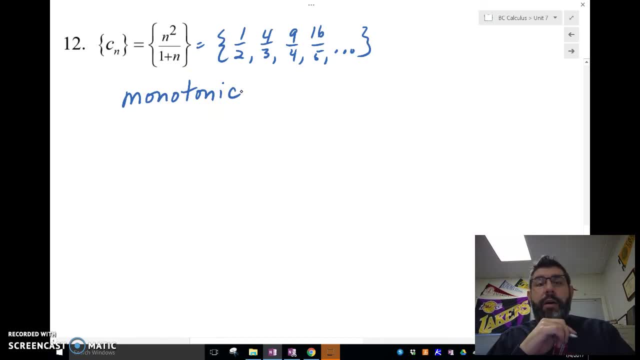 monotonic. okay, however, um. one half, four, thirds, nine, four, six, 16, fifths and so forth, um, it's bounded below, it's about- and i'm going to write this here in red here, um it's. it's bounded below um by one half, right, because one half is the lowest it's going to be. 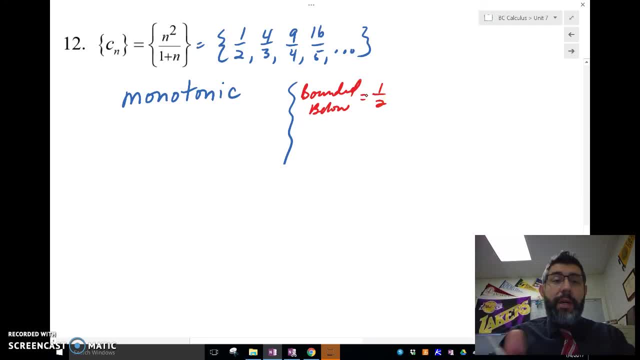 but as it gets bigger, it's going to keep getting bigger. this n, squared on top, is going to- if i took the limit as an approach- infinity. i'm not going to approach anything. it's just going to keep getting bigger and bigger. so it's not bounded above. so we're going to say that this function. 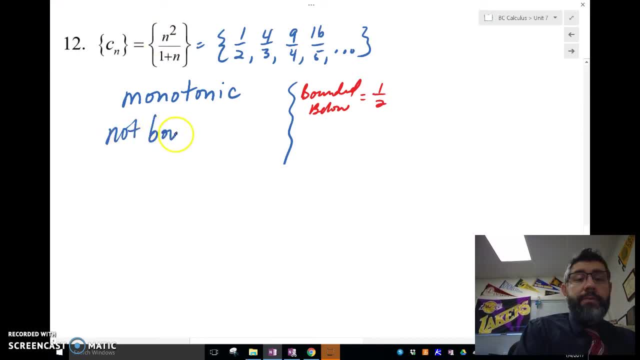 is, we can either say it's not bounded or we can say unbounded, oops, um, it is bounded below but it's not bounded above. and in order for some, for a sequence to be bounded, it needs to be bounded above and below. and you know what, guys? i'm sorry if i kept. 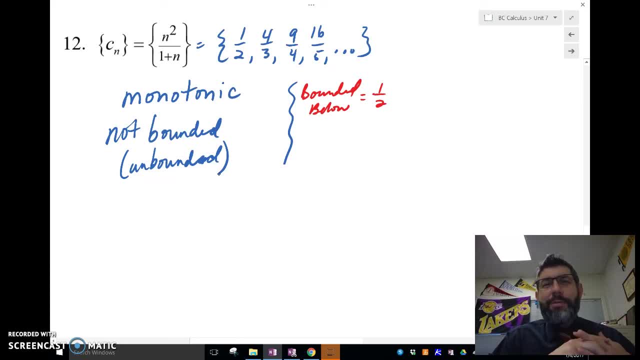 saying function. i should not be saying function. i don't know why i'm saying function. um. don't say that we're not dealing with functions. we're dealing with sequences. um, and this right here, this is the explicit formula for the nth term of that sequence. we're dealing with sequences. 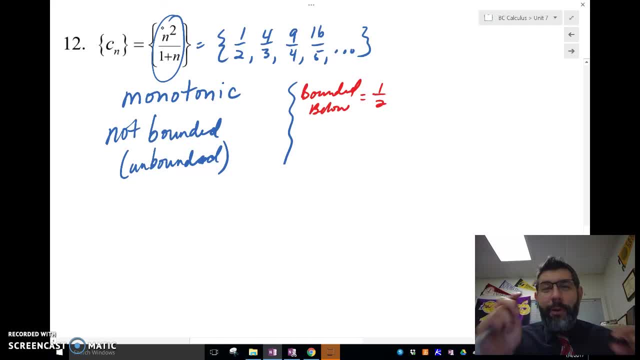 so if i said function, i am sorry. erase that from your memory gone. we're talking about sequences, all right, okay, so that's the end of our sequences. we're going to take our questions. we're going to get them on on our end of the day, but first i want to thank you all so much for watching and see you. 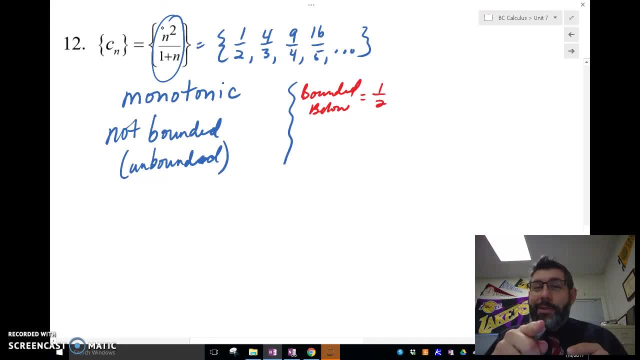 back next week. our next video is fun, so stay tuned. bye-bye. bye-bye this video. We'll see you soon, Bye.